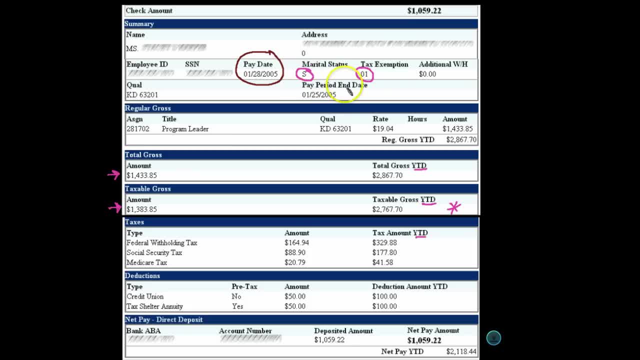 because depending upon how many exemptions you claim, the combination of that and your marital status- whether you're single, married, head of household- that'll change how much is withheld for federal tax purposes. Then I have the pay date here, or the pay period. 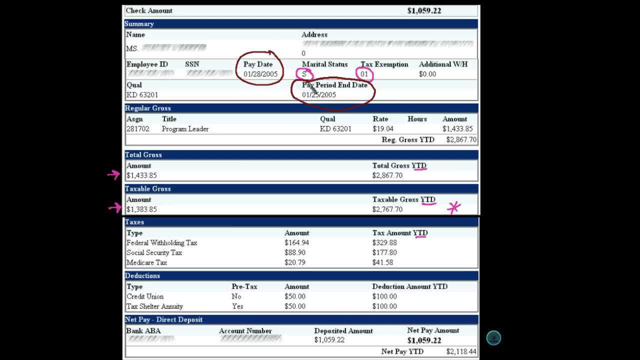 end date. This is going to be important because you'll need to know how many times you've paid, how many times a year you're going to be paid if you're going to make an estimate Couple. other things that are important are total gross and taxable gross Back in quarter. 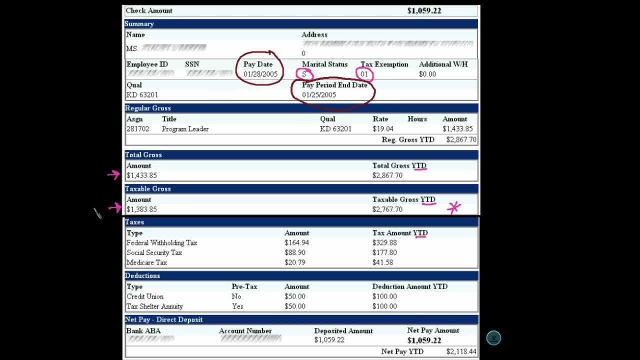 one. we talked about total gross and we talked about net pay. Down here at the bottom you can see your net pay. You learned that the net pay is what you actually bring home in your pocket and the gross pay is what you actually earned. You never really get your. 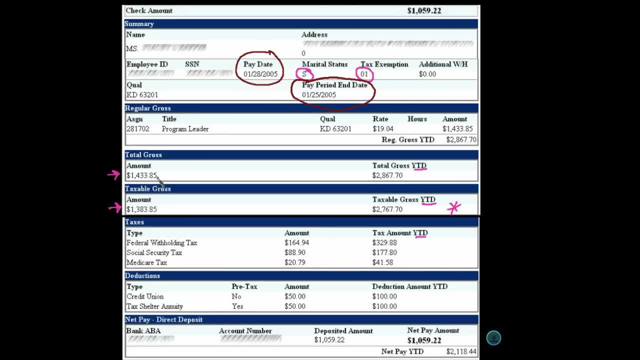 gross pay, because you're always required to pay some taxes like Social Security and Medicare. Now we have this extra category called taxable gross. The taxable gross is what's reported to the IRS as far as the amount of your income that's taxed. Notice that, even though you 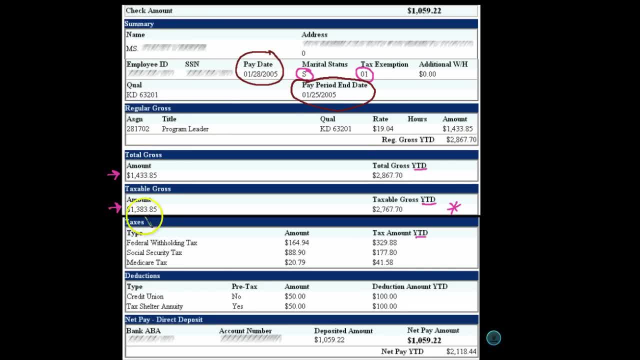 earned over $1400, you're only taxed at 13-something. Part of that amount that you earned is not taxed. Why is that? Well, employers often have retirement plans. If you contribute money to a retirement plan, that money can come out of your income before the rest of your. 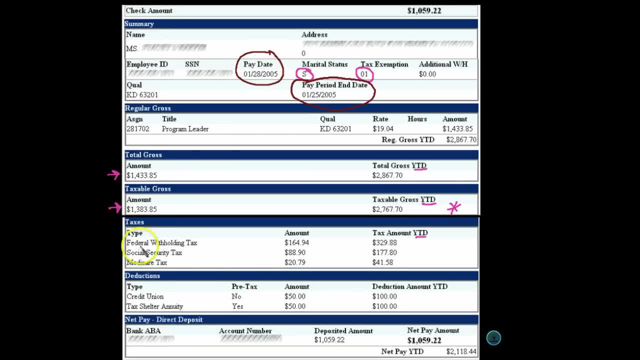 income is taxed In this case. if we look down here at the bottom under deductions, we have a column here that says pre-tax yes or no. Well, in this example this employee is contributing to a credit union $50 for something. That amount is not pre-tax. But 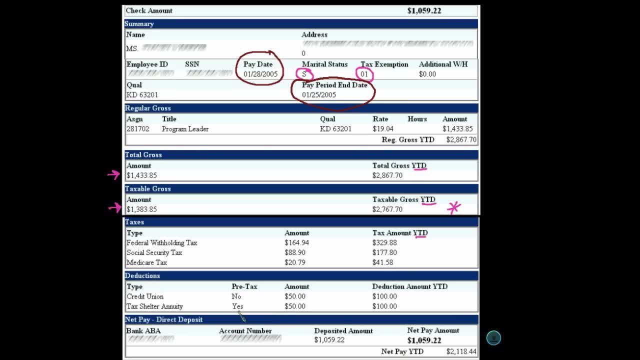 then we have a tax shelter annuity and that is pre-tax And, if you'll notice, that amount is $50.00.. The difference between $1433.85 and $1383.85 is exactly $50.00.. So this employee is having 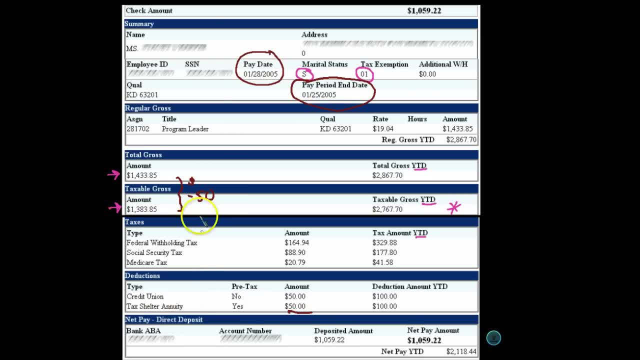 $50.00 put into a retirement plan. that is not taxed. There are sometimes other things that are not taxed. If you contribute premiums to health insurance or dental, there's sometimes an option to have those come out. But if you contribute premiums to health insurance or 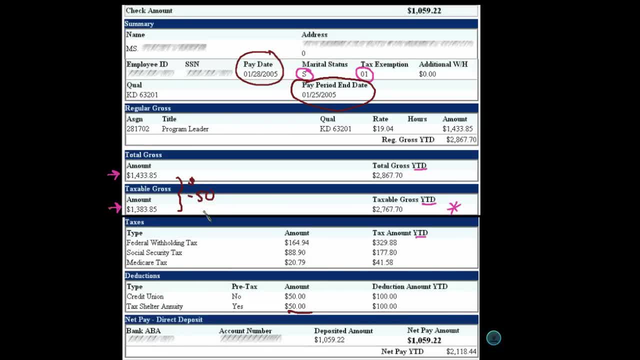 dental, there's sometimes an option to have those come out. But if you contribute premiums to health insurance or dental, there's sometimes an option to have those come out. But if you pre-tax as well, Okay, a couple other things, then. that we need to notice is: 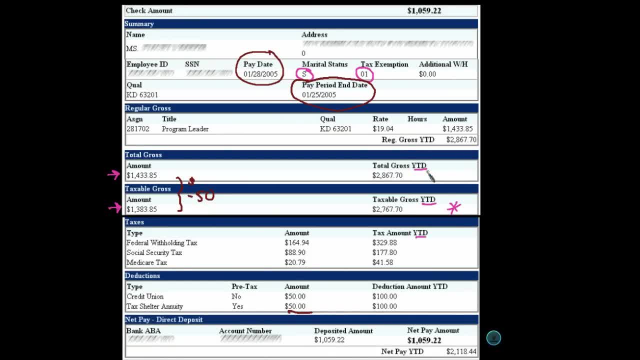 that in this column on the right is: we have a year-to-date, So this is what we have earned year-to-date. Notice that each paycheck amounts to about 1433 and we have earned a total of 28.. So that means this is only our second paycheck. of the year. Our pay period ends January 25th, So how is this employee being paid? He could be paid twice a month, which would then mean that there are 24 pay periods for this employee, or he could be getting paid every other week. Well, 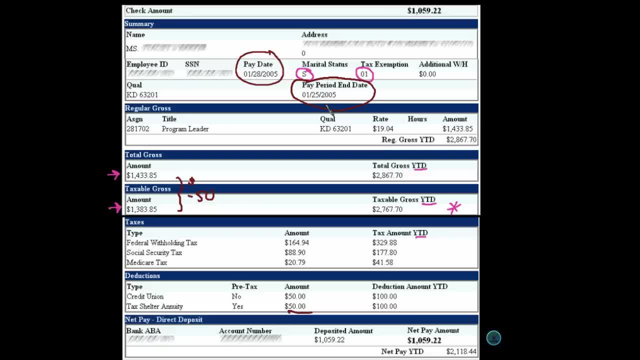 there's 52 weeks in a year, so that would then be 26 pay periods. Well, based on the fact that the period end date is the 25th, I would say he's probably being paid every other week, and so in this case we'll say that he has 26 pay. 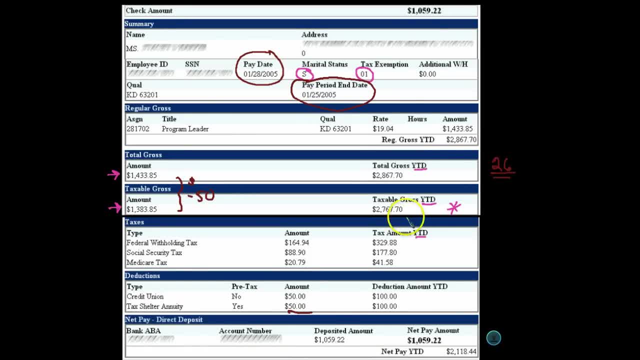 periods. That's going to be our pay period for this employee. It's going to be important when we are calculating or projecting what this employee will make by the end of the year. We also need to look at our tax amount. We're especially concerned with our federal withholding. We need to know. 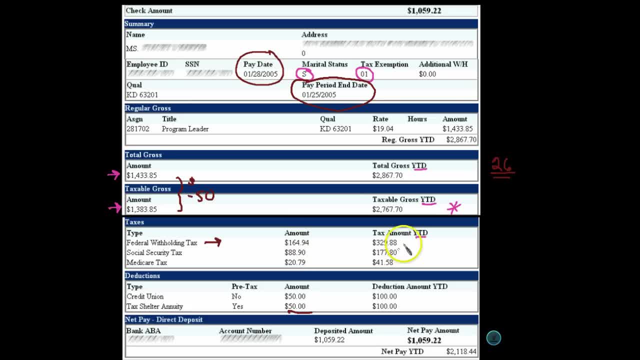 how much is being withheld every paycheck and how much has been withheld so far. We don't care about Social Security or Medicare. Those are required and we're not taxed separately other than what our employer takes out of our paycheck. All right, I think that's it for today. Thank you so much for watching. I'll see you next time. 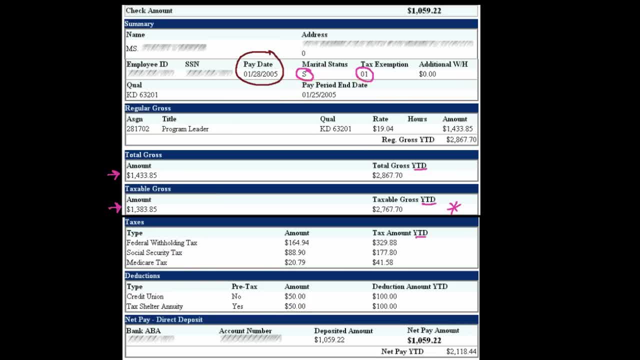 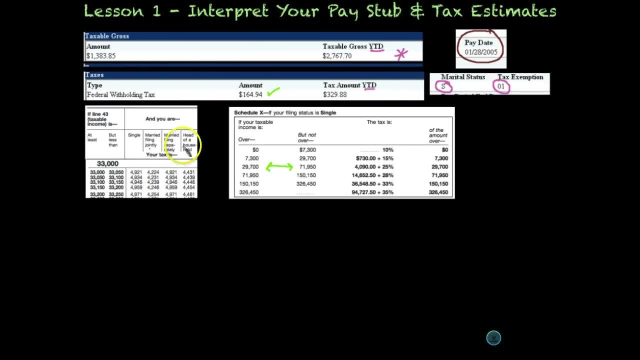 For Rady. let's go ahead and do some quick calculations. What I've done is I've pulled some key pieces of his paycheck or pay stub off onto a separate area for us. Here's the amount of his taxable gross and his year-to-date taxable gross. 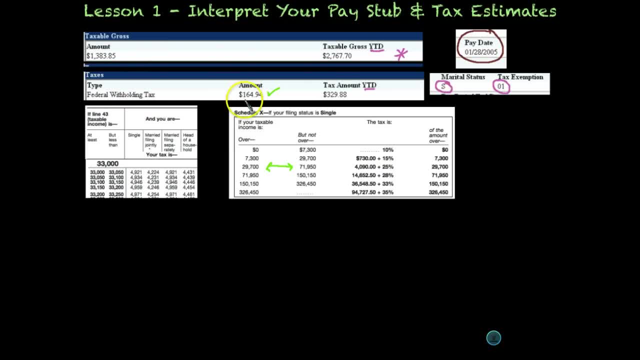 We also have the federal tax withholding amounts for this check and the year-to-date amount. We know that the pay date was January 28th, but that is pay period ended January 24th and we said that there are 26 pay periods in the entire year for this person, but that he's already been. 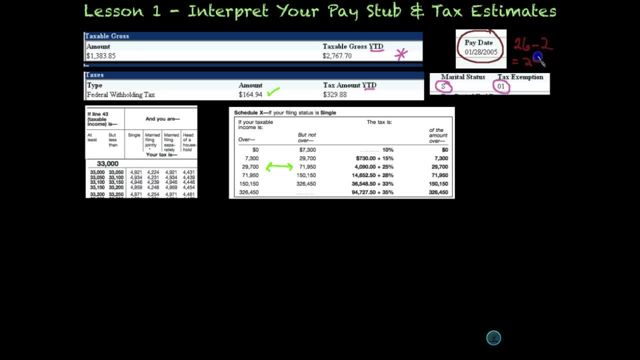 paid two, so he has 24 pay periods remaining. This person is single and claims a tax exemption of one. That's informational, So I've pulled here a single schedule for this year Over. here is just a screenshot of a tax table. Remember that we can use either or. 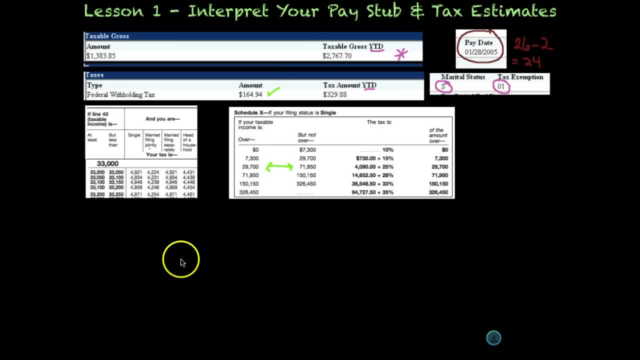 In the back of your tax instruction booklet when you go to fill out your taxes. you will see both and you can choose which one you'd like to use. We're going to go ahead and use the schedule and do a calculation, but remember that this is always an option as well. All right, in order to determine and make an. 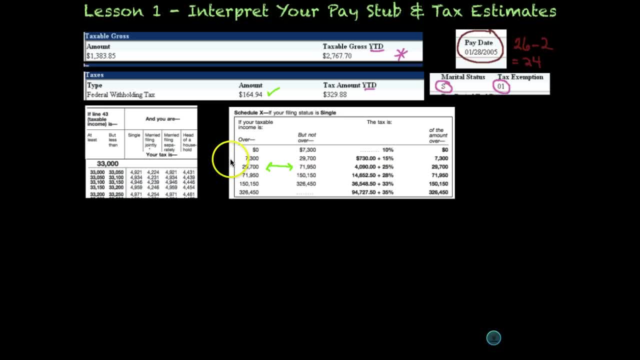 estimate for our federal tax liability each year. we need to start with one determining how much we're going to make and two determining how much is going to be paid. Let's start with step one. Let's find this person's total taxable income for the year. So we look at our taxable gross and we look at our taxable gross year to. 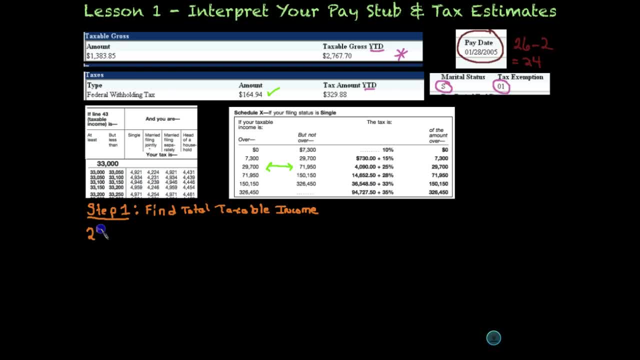 date. So, no matter what, this person has already earned twenty seven, sixty seven, seventy, but we need to add to that thirteen, eighty three. This is what they make per pay period Times the number of pay periods left. We just said there's probably twenty four pay. 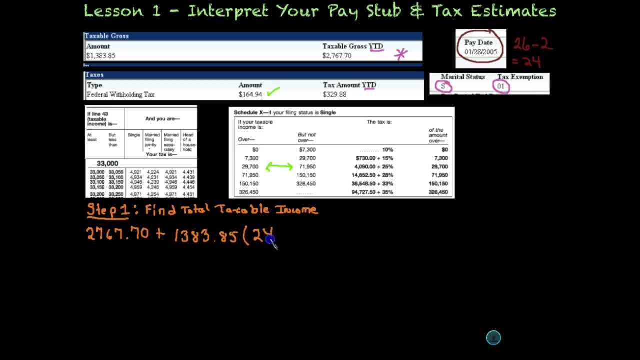 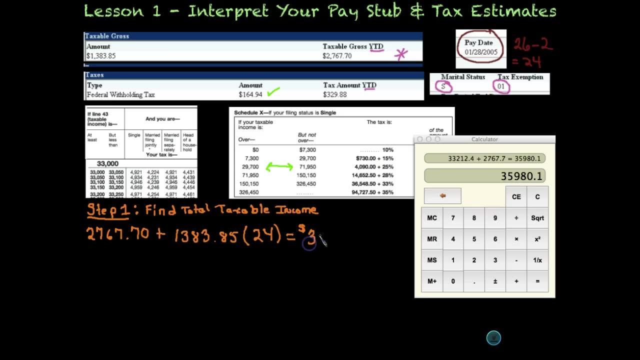 periods, because we're assuming this person gets paid every other week. Alright, once we simplify this, we will have this person's total taxable income. When I put this in the calculator, I get a total income of thirty five thousand nine hundred eighty dollars and ten cents. 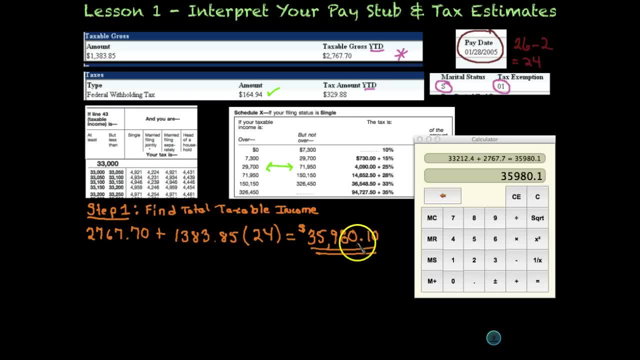 That is, this person's projected taxable income in a year. Alright, let's move on to step two. In step two, we're going to estimate how much federal tax is going to be withheld, based on the tax exemption that this person claims and the marital status. 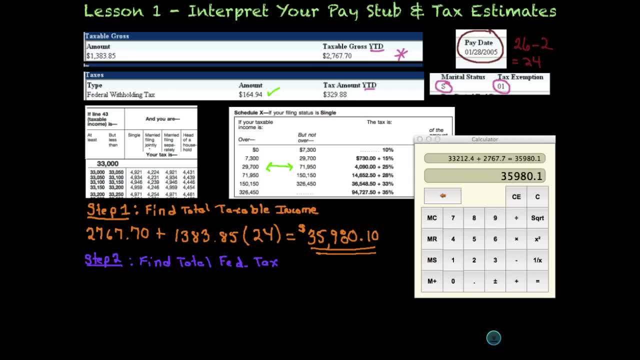 Well, so far he has had three twenty nine eighty eight withheld, so we can include that Three twenty nine eighty eight plus. this person has a hundred and sixty four dollars and ninety four cents withheld and we've determined that each pay period- and we've determined there's 24- remaining pay periods. Okay, again, simplifying this, in the calculator we get total projected tax withholdings of four thousand two hundred eighty eight dollars and forty four cents. The question is then based on a projected income of almost thirty six thousand. is this amount of federal tax going to cover it? What is this person? 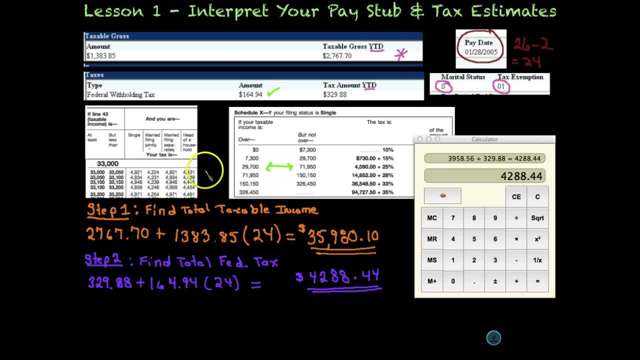 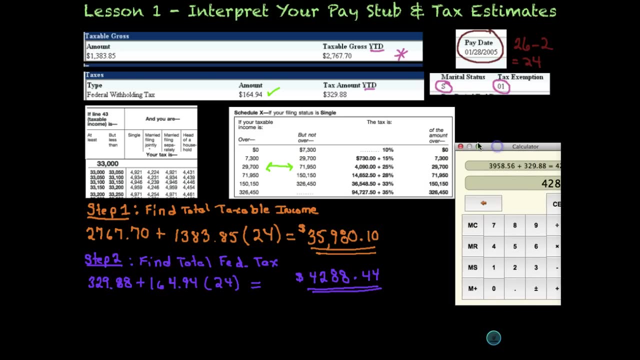 going to owe. That's where our tax schedule and tax tables will come into play. Notice that I put a green arrow here under this category. If this person is projected to make thirty five thousand nine hundred eighty dollars, that's going to fall in here. So if that's the case, then we 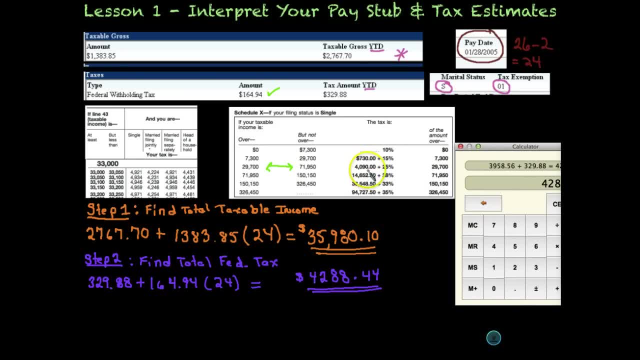 know that he is going to owe or she four thousand ninety dollars, plus twenty five percent of any amounts over twenty nine thousand seven hundred. That then brings us to step three. We need to calculate this person's tax liability, Using the table to help us make an algebraic expression. we know they're going to owe. 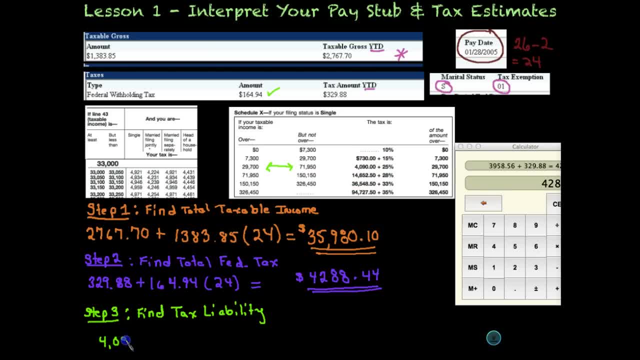 four thousand ninety plus twenty five percent of the amount over twenty nine thousand seven hundred. Well, we're projecting this person will earn thirty five thousand nine hundred and eighty, and I'm going to round, I'm going to leave off this ten cents. it's immaterial and insignificant. 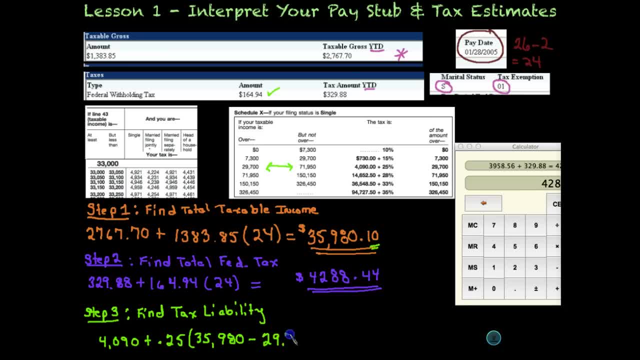 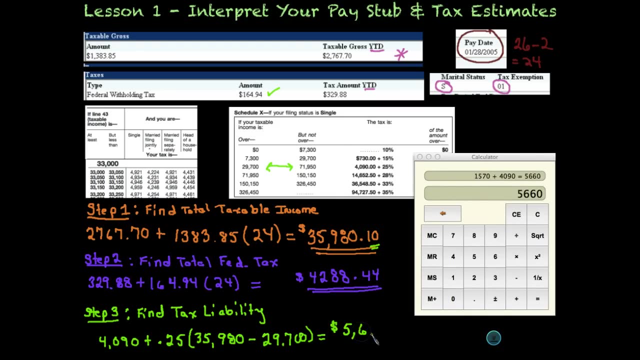 and then I'm going to subtract the twenty nine thousand seven hundred. Okay, in my calculator I'm going to subtract these, multiply by 0.25 and then add four thousand ninety. When I do that, I get a tax liability of five thousand six hundred and sixty. 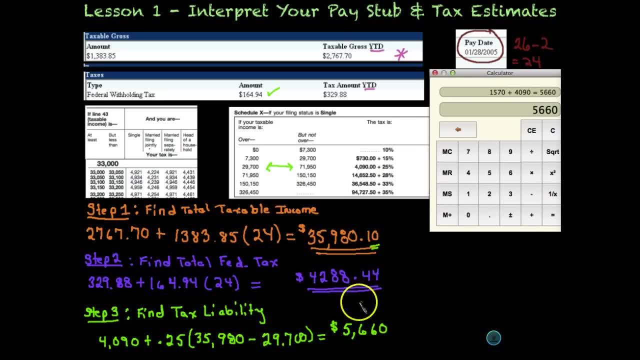 Well, that's definitely more than the projected amount that he will have withheld, but how much more? So let's do this: Let's go ahead and subtract the amount that's projected to be withheld and again, I'm going to just round and take off the forty four cents minus forty two, eighty eight, and I get. 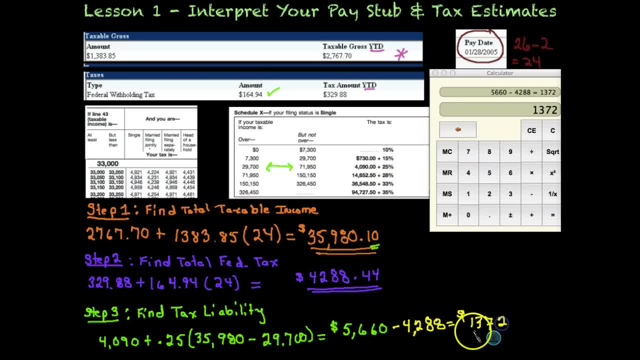 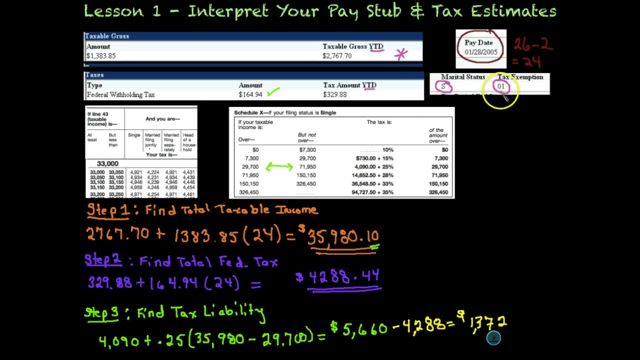 thirteen seventy two. So for this person, they would have to think: is thirteen seventy two a reasonable amount to have to pay the IRS April fifteenth? If it seems like a lot, then this person needs to change their exemptions from one down to zero, and we're about to talk about that. Or if this seems okay, then this: 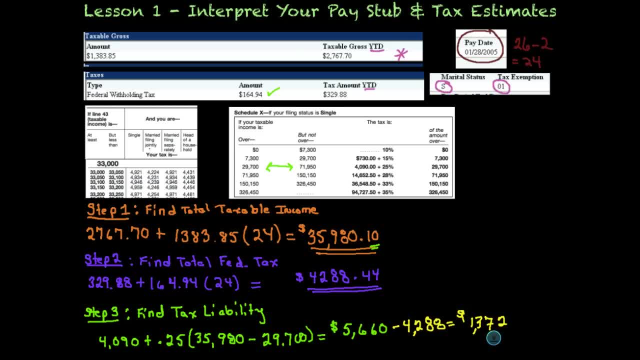 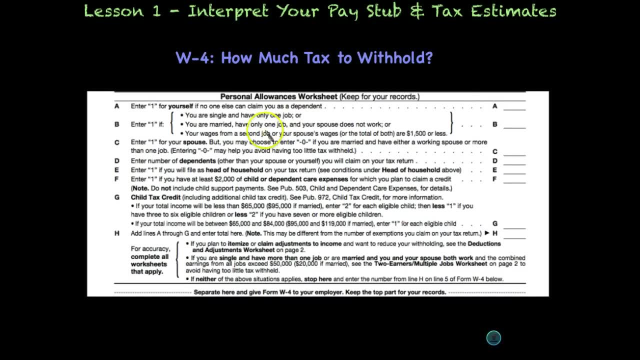 person is on track. So let's go ahead and look at how we do that. Whenever you start a new job or change your job, You can do it at any time. on your current job, You fill out a personal allowances worksheet to help you fill out your W-4.. 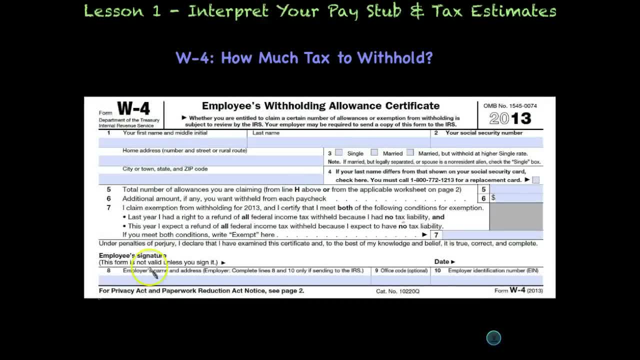 Your W-4 looks like this: Notice that you put in all your personal information and then, starting here at line 5, total number of allowances you are claiming, And then it says from line H or above, or from the above applicable worksheet: 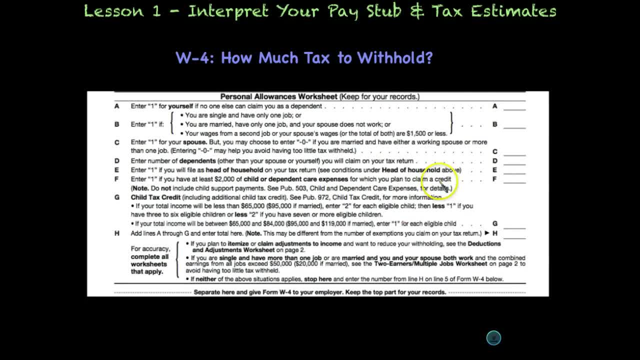 Well, that's this worksheet. You can choose to fill this out or you can just make a rough estimate of how many exemptions you'd like to claim. So, the one thing that you have to keep in mind- and this is where people often have confusion- 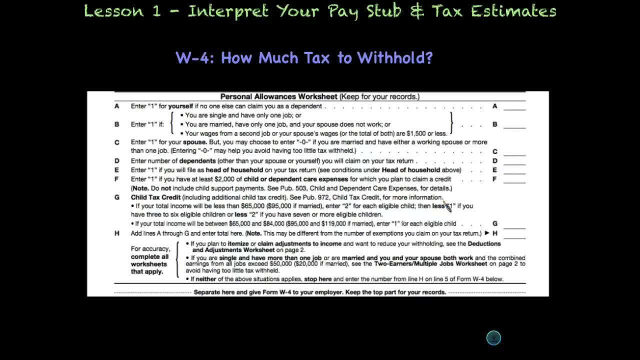 if you claim zero allowances or zero exemptions, you are going to have the most amount of federal tax withheld from your paycheck each pay period. The more allowances or exemptions you claim, the less federal tax you're going to have withheld. What is an allowance, What is an exemption? 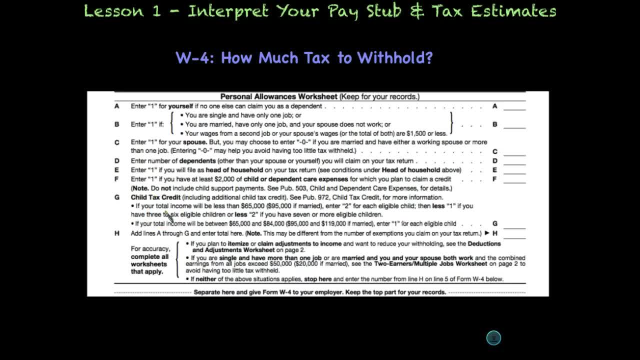 Well, notice here. this worksheet helps you to think about that. You automatically get one exemption for yourself. You also get one if you're married and only have one job, your spouse doesn't work or your wages are fairly low. You also get a one for your spouse if you're married. 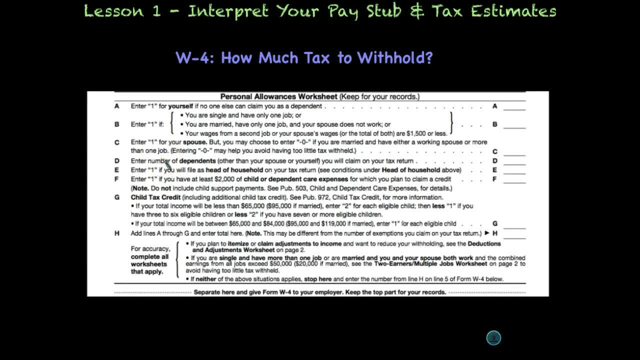 You get ones for your dependents. If you have two children, you get two. There are other things on here, too, that increase your exemptions. In the end, when you add up all the exemptions you list here, that becomes your total exemption. 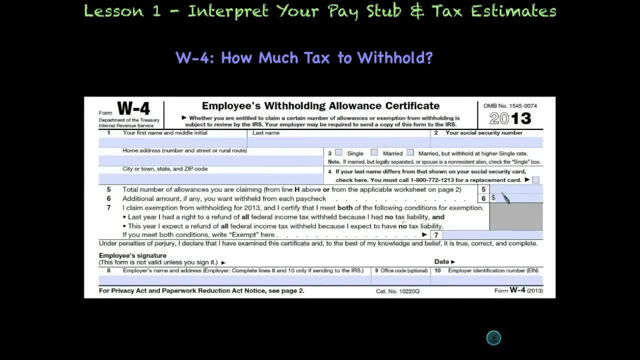 which then you put over here on line five. All your employer cares about is what you put on that line five. So if you put ten exemptions, your employer is not going to withhold very much federal or state tax. If you put zero, they're going to withhold more. 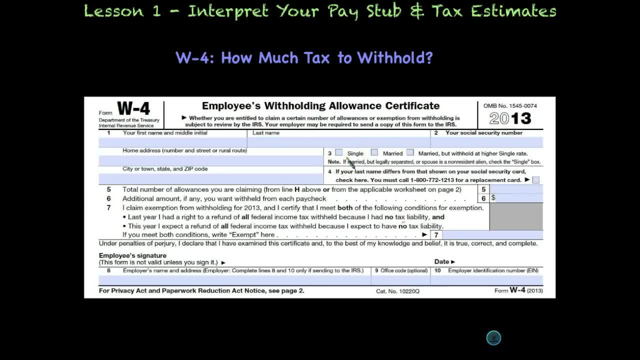 Your filing status matters too because, remember, there's different tax rates depending on if you're single, married, married, filing joint. So if you put single or married with the zero, it's going to be a different amount: Single if you are single, with zero withholding. 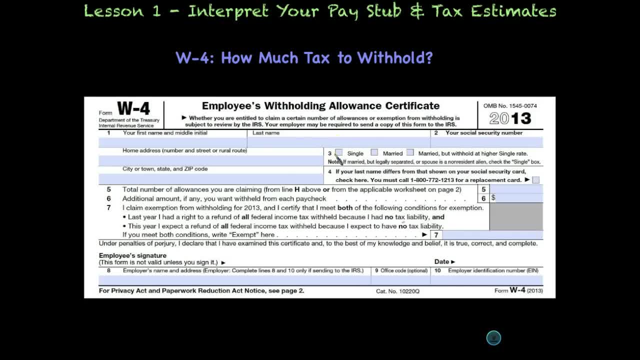 that's the maximum amount that you can have withheld. If you put married and then you put ten, not much is going to be withheld. There is this box seven. here You can claim an exemption. Most students claim this, So you can write exempt here. 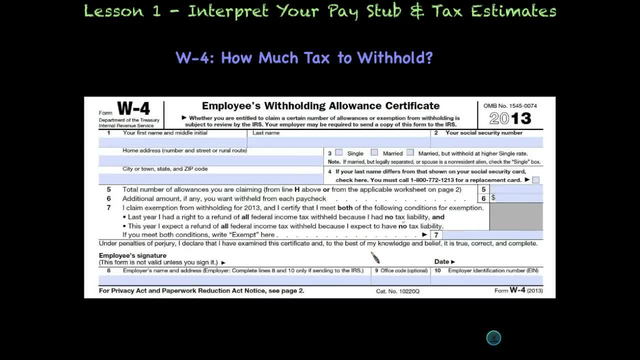 and that means no federal or state taxes will be withheld. There are two conditions for you to be able to claim exempt. Number one: last year I had a right to a refund of all federal income tax withheld because I had no tax liability. So the key is no tax liability. 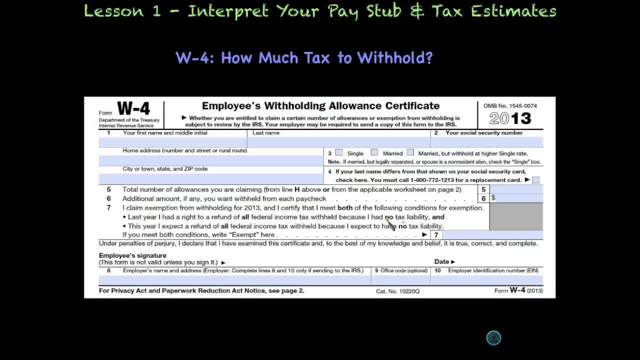 And this year I expect a refund of all federal income tax withheld because I expect to have no tax liability- And you're probably wondering how it is that you could have no tax liability- And we'll look at how the federal income tax return works in the next couple lessons. 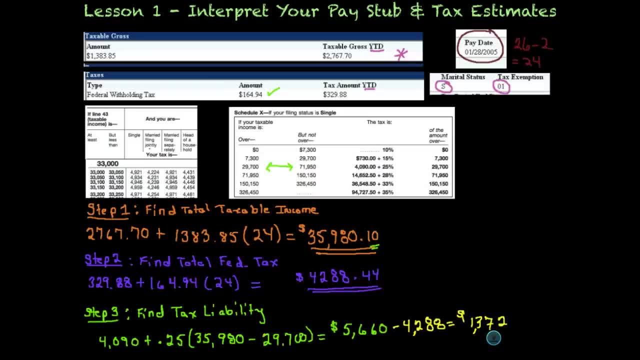 But basically, if we go back to our example here with our taxpayer, we just assume that his taxable income is what he would be taxed on. But when you're filling out your tax return, there are certain things that you can also deduct from that. 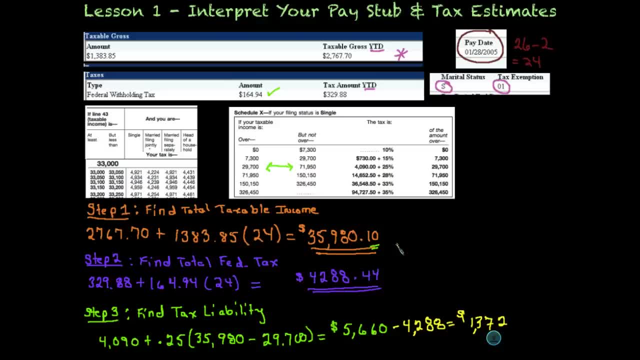 to come up with your adjusted gross income And we'll be exploring some of those deductions. But just for an idea, if you have children, you get extra exemptions. If you own a house, you also get extra deductions. So this $35,000 is a conservative number. 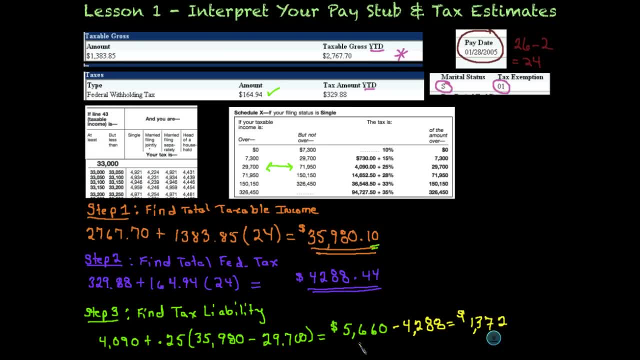 This tax right here, $5,660, would probably be the most that this person would owe based on this income. In fact, this person would probably owe a little bit less, Alright, that concludes our lesson today on interpreting your pay stub and making some tax estimates. 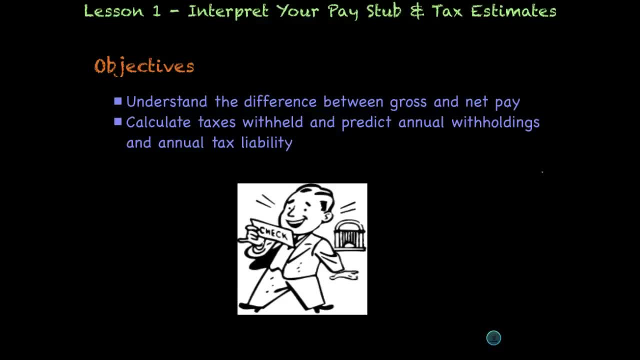 So again, remember to be successful. after this lesson, you should be able to look at a pay stub, find the taxable income or the taxable gross income and then use that in conjunction with the pay stub, And then use that in conjunction with the pay date. 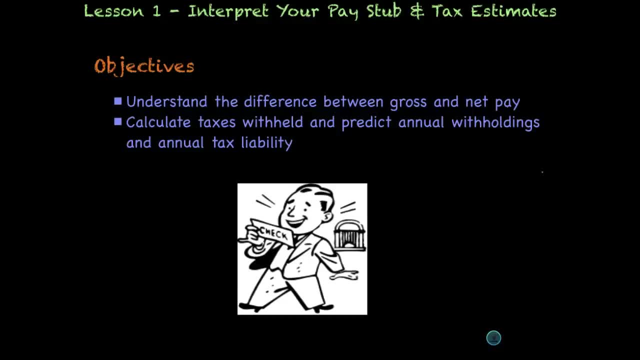 and the amount withheld year-to-date to determine or predict your total income at the end of the year, as well as do the same thing to predict and determine your federal income at the end of the year, And then use that information in conjunction with your understanding.